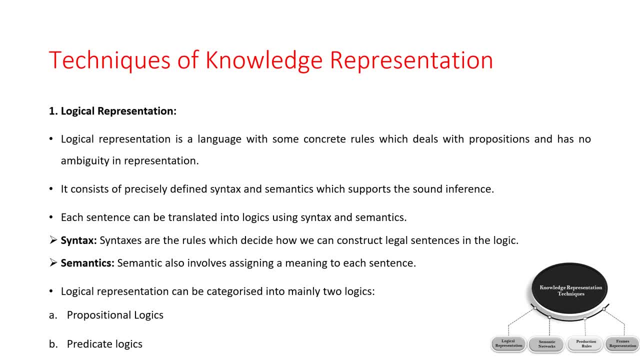 rules, which deals with the proposition logic and has no ambiguity in the representation. ambiguity means what non clear, so no ambiguity means what: whatever the meaning is, whatever the knowledge is, its meaning should be clear, so it has no ambiguity in the representation. so logical representation means: 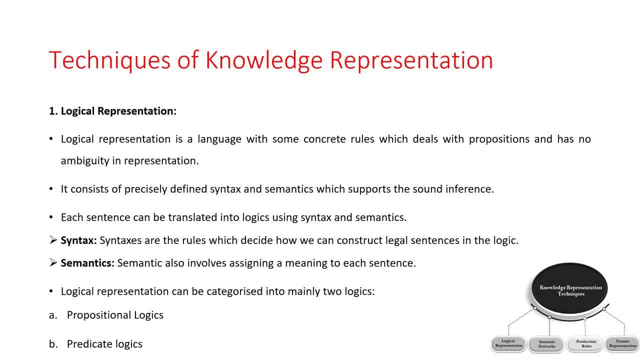 drawing a conclusion based on the various conditions. we are having some statements. based on the statements, we have to provide some conclusion based on the various conditions. so this representation lies down some important communication rules. so it consists of precisely defined syntax and semantics which supports the sound inference. 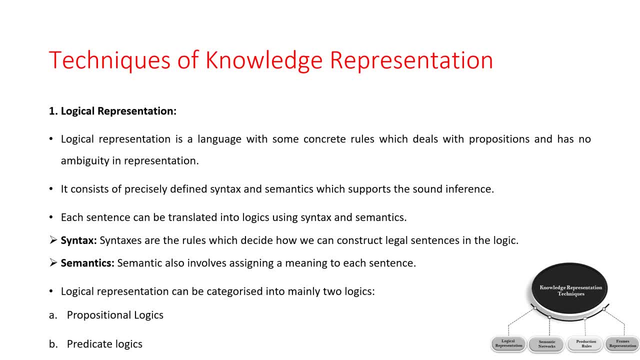 so each sentence can be translated into the logics using the syntax and semantics, if we have any sentence, if we want to get the conclusion or if we want to represent it properly. so there should be no ambiguity in the sentence. meaning should be clear. so whatever sentence we have, 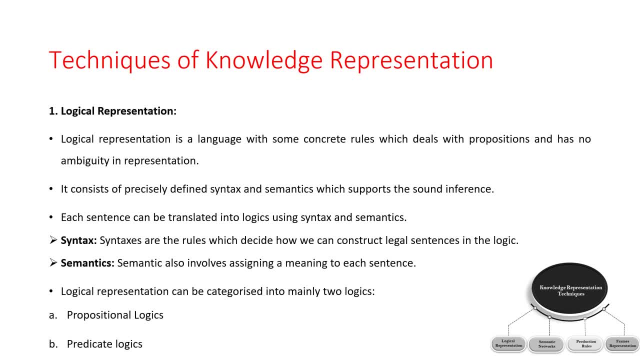 can be used in two forms, so we should check its syntactically and semantically. so syntax means what syntaxes have the rules which decide how we can construct the legal sentences in the logic. so this syntax says determines which symbols we can use in the knowledge. 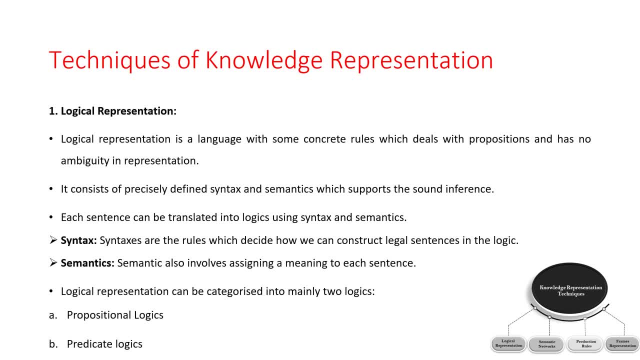 representation, if we want to represent any sentence in the knowledge, so which syntactically symbols we should use and how to write those symbols. and how to write those we should know. and the next thing is semantics. what is meant by semantics here? semantics are the rules by which we can interpret. 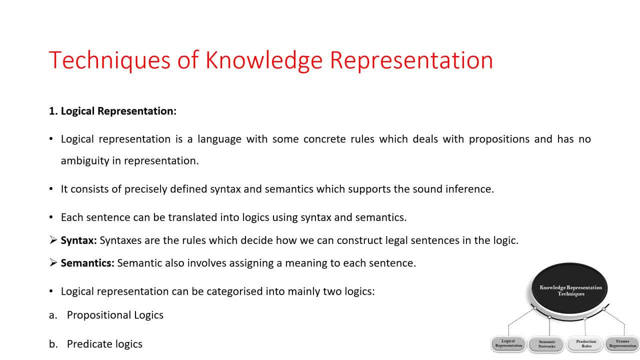 the sentence in the logic, how we will interpret our sentence. so this is all about the semantics. semantics are also involves assigning the meaning to each sentence. we have only one sentence, if we want to check its syntax, if we want to check its symbols, so this is all about syntactically. 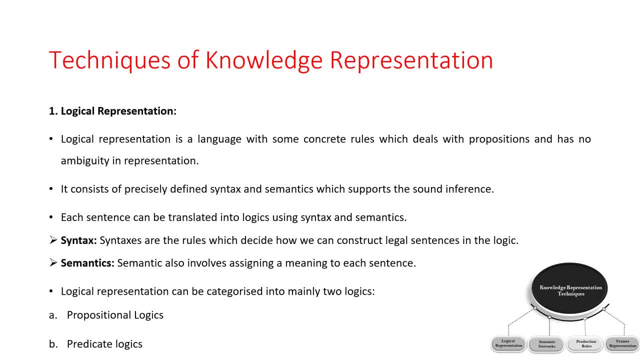 and whatever sentence we have, if we want to check its meaning, what is clear, if we want to check that. so this is semantically so. logical representations can be characterized into the mainly two logics. first is the proposition logic and the predicate logic. so in the next lecture, 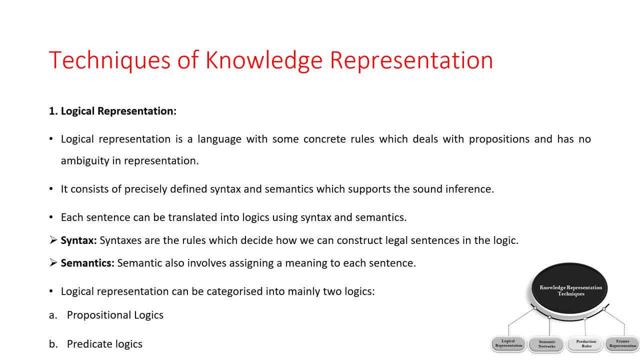 we are going to discuss about what is mean by proposition logic, how we use this proposition logic, examples of proposition logic and the predicate logic also. so in this video we are going to only discussing about the techniques of knowledge representation. so these things we discuss in details in the 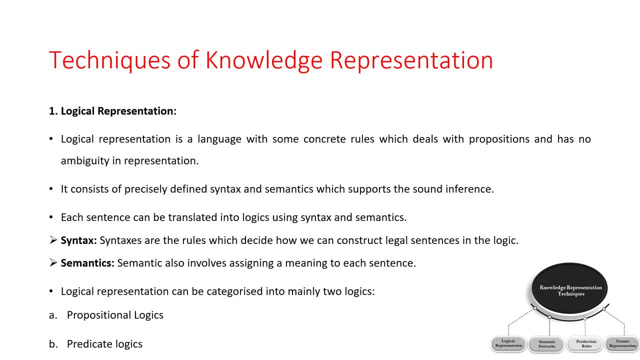 next videos. so what are the advantages and disadvantages of this logical representation and when we use this logical representation? so advantages of logical representations are we can enables us to do the logical reasoning. logically, we think if any sentence comes to us, if we provide any sentence to a human, 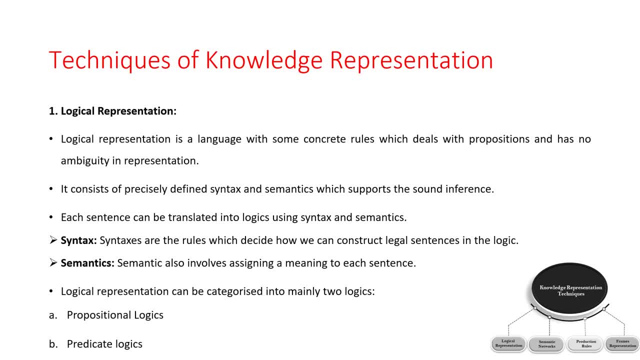 then we think logically that what will be the meaning of this, what we have to do in sem, we have to train the machine like a human. that what will be the sentence after that, how it will represent logically, so in the form of proposition logic or in the form of predicate logic. 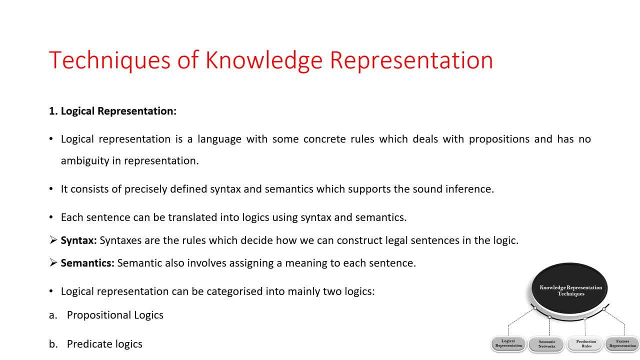 if I get any statement that if the rain, if the rain is come, then the road is a wet. when it will rain, when it will rain, then our road will be wet. so this sentence is true. we will know easily that if it rains, then our road will be wet. 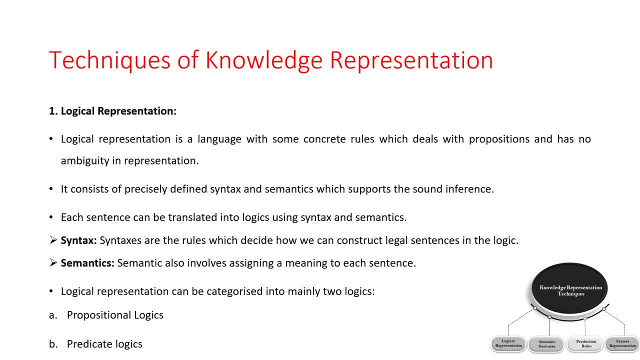 ok, so this statement, human can easily understand that this particular statement is true. if I consider any other statement like hot ice cream, ok, so this statement is true or false, human can easily understand that this particular statement is false. ok, so we put the logic here that whatever sentence we get, 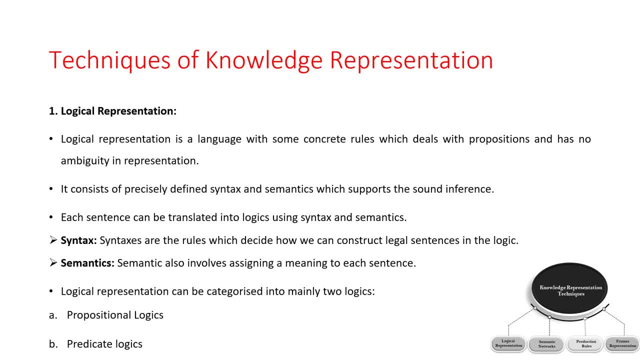 is it logically correct or not? is it true or false? ok, so human can easily understand, but how machine can understand? ok, so this is all about the logical representation. so what we have to do with machine, whatever knowledge it has, we have to represent it. for that we use techniques. 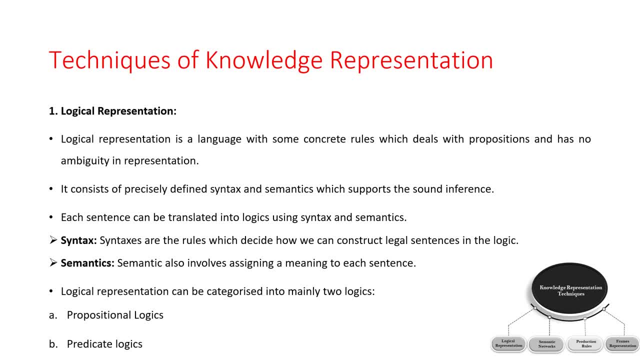 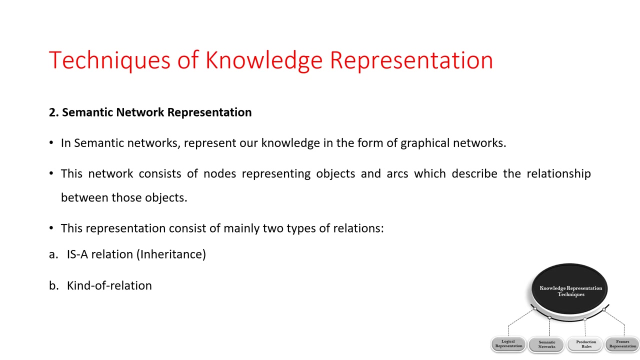 logical representation. ok. so the second advantage is the logical representation is the basis. is the basis for the programming languages? we can represent it with programming languages, ok. so this is a first technique of knowledge representation, that is, the logical representation. the second technique of knowledge representation is the semantic network. 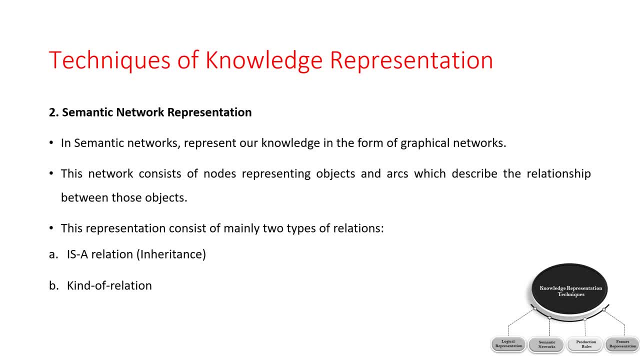 representation. so semantic networks are alternative of predicate logics for the knowledge representation. ok, what is the alternative for predicate logic representation? so in semantic network representation we can represent our knowledge in the form of a graphical network. so this network consists of nodes representing the objects and arcs. 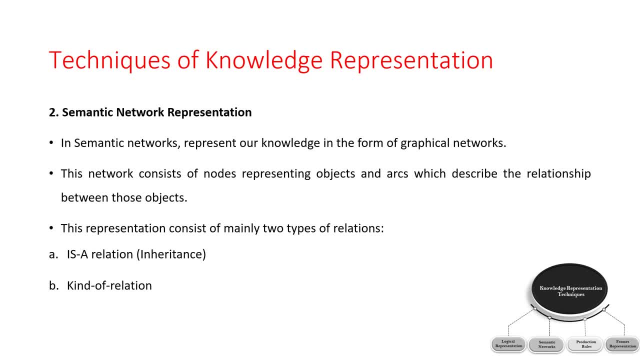 which describe the relationship between the objects. ok, so if i have two objects and i want to show the relationship, then i will use arcs which will show the relationship between two objects. ok, so semantic network can categorize or categorize the object in a different form and can also link those objects. ok, so semantic network are easy to understand. 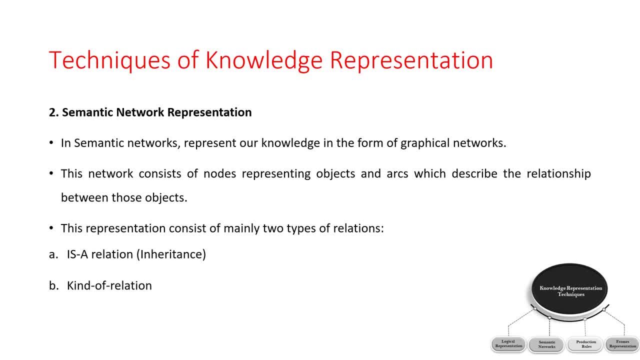 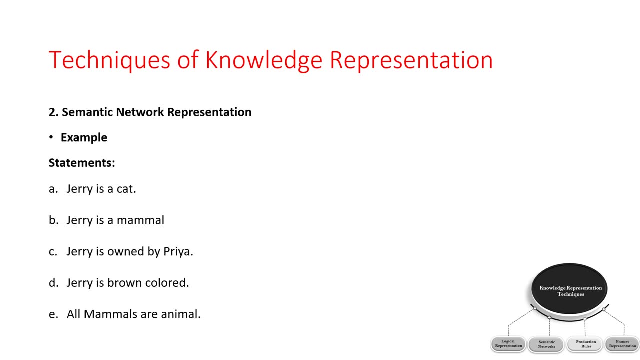 and can easily extend it. so in the semantic analysis or network representation, there are mainly two types of relations: is a relation that is called as inheritance and the kind of relation ok. so see, here there is one statement, ok. so this is a simple example related to this semantic network representation. so there are some statement which we need to represent. 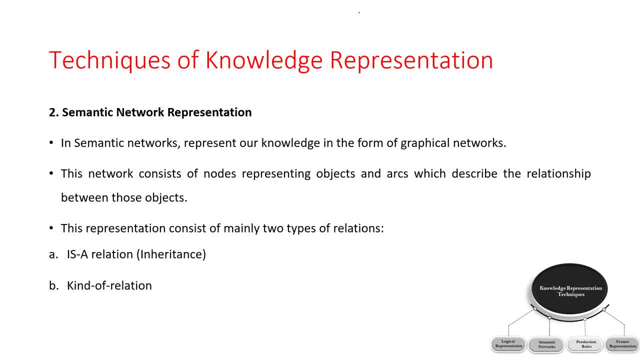 in the form of a node and arc. ok, as i have explained, in semantic network We can use objects and objects from graphical networks to represent it. If we have a graphical diagram so the user can easily understand what is the relation between them and how it will happen. 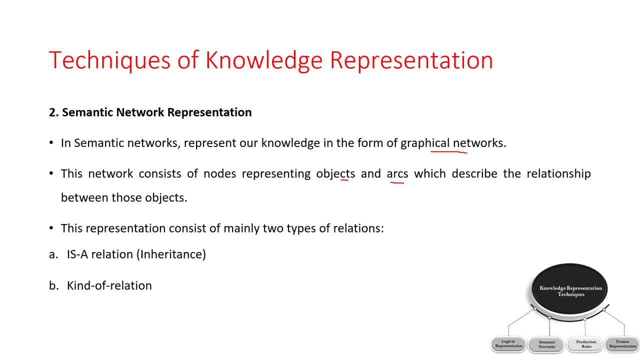 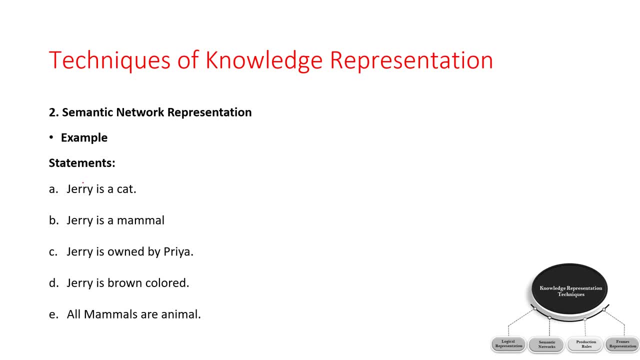 So we have to provide the same machine with representation. We have to provide the same machine with representation in the form of a graphical. So if we have some statements like Jerry is a cat, Jerry is a mammal, Jerry is owned by Priya, Jerry is brown colored and all the mammals are animals, 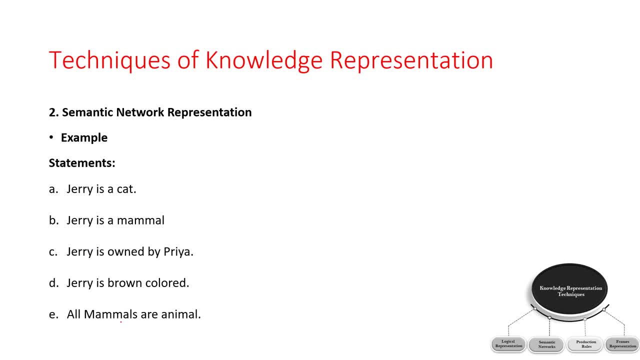 So we have to represent this statement in the form of nodes and arcs. So we have a common statement, Jerry. So here I have created a node which will be our object Jerry. Jerry is a cat, So here I have shown E as a relationship. 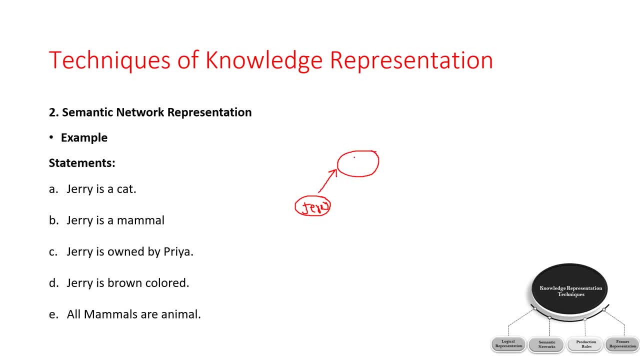 Jerry is a cat, So Jerry is one object and cat is another object. So here I have shown E as a relationship, So E is a relationship. The next is: Jerry is a mammal. Jerry is a cat, Jerry is a mammal. 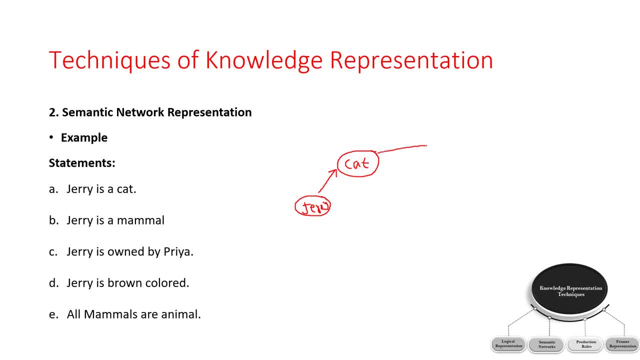 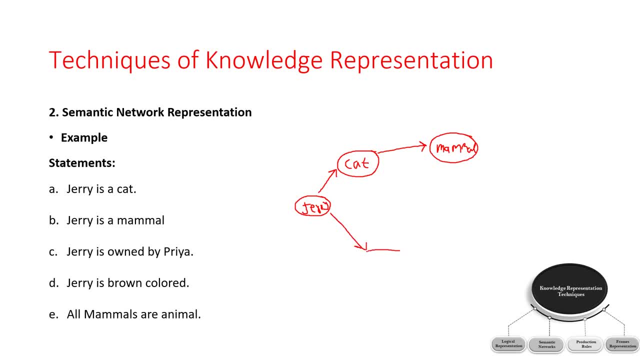 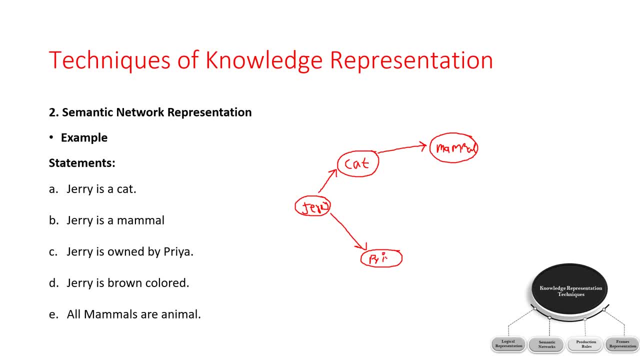 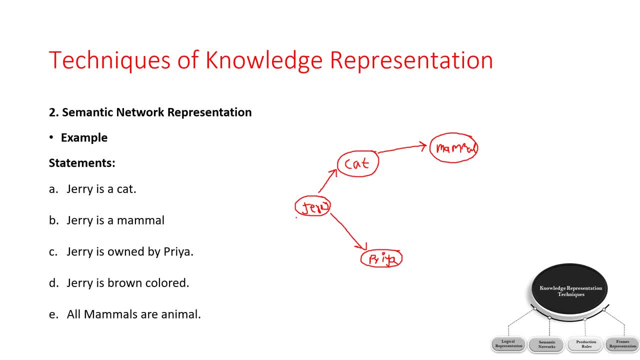 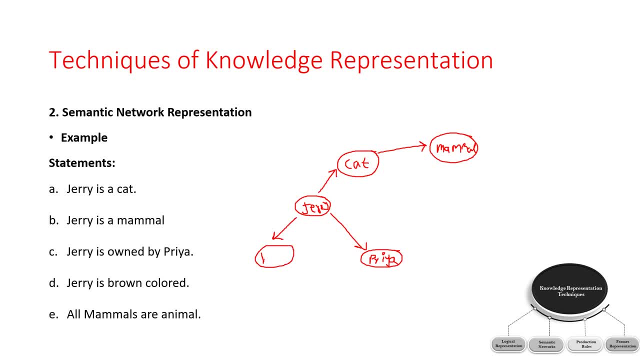 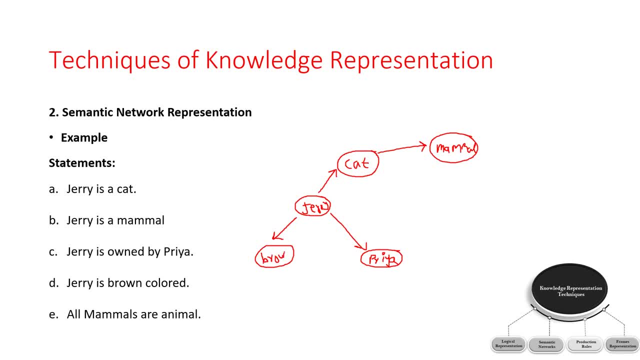 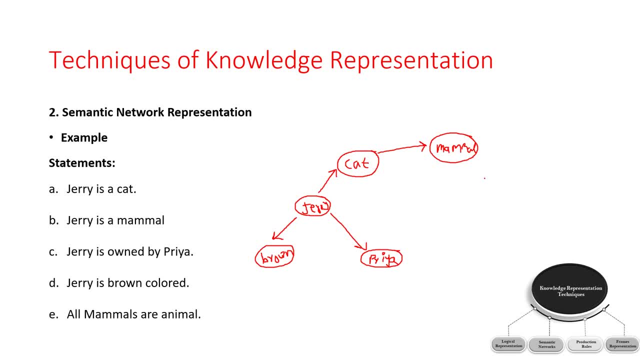 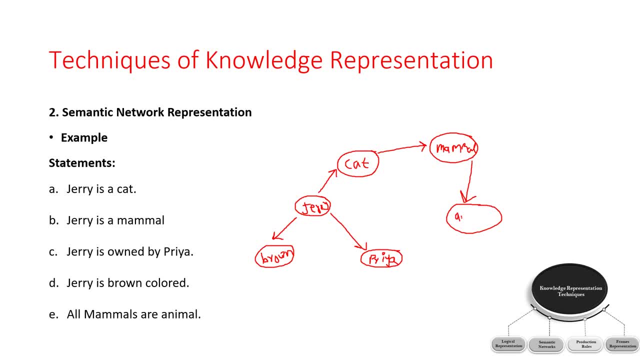 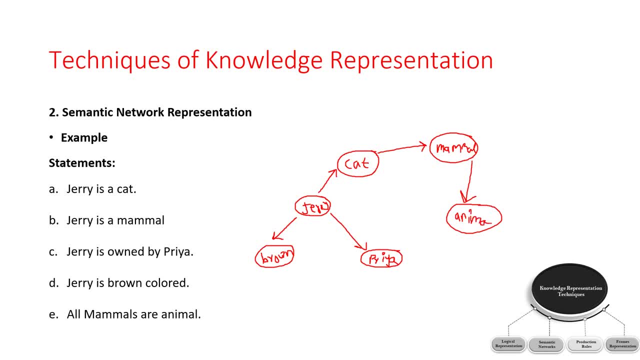 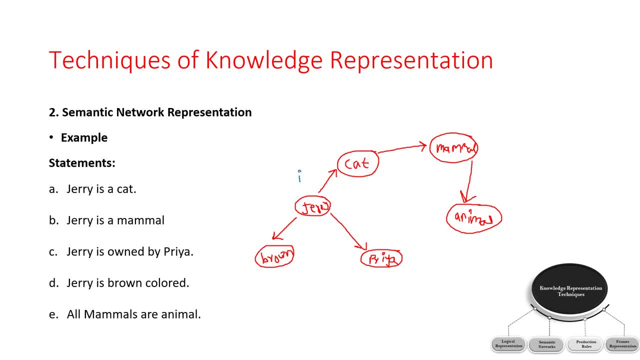 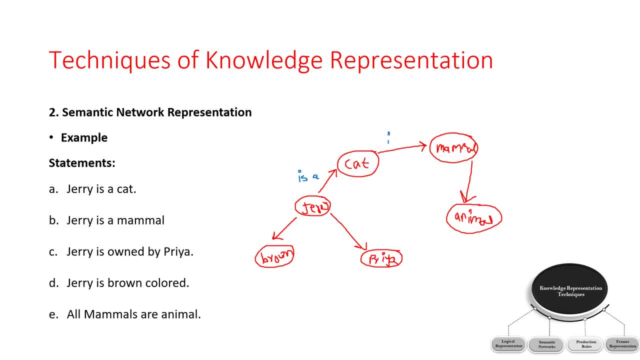 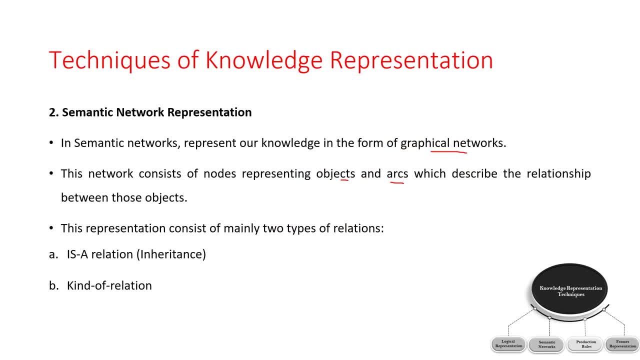 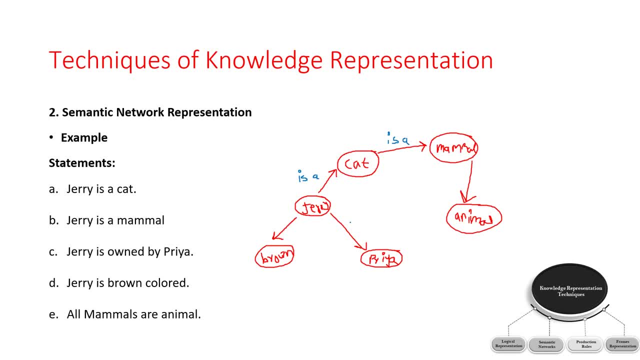 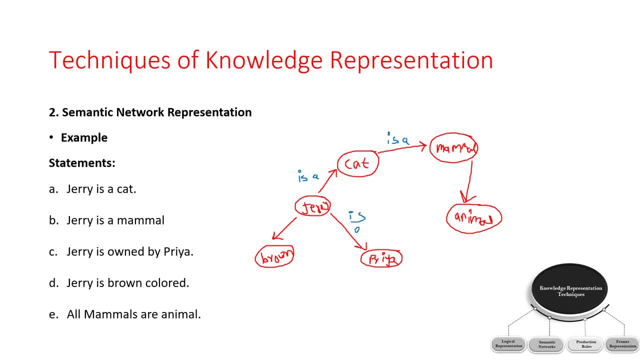 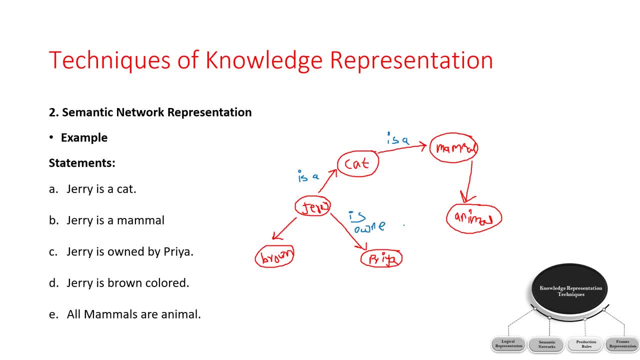 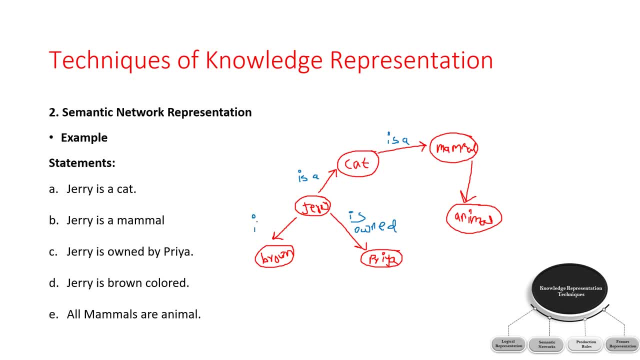 He's colored. So Jerry is a brown color, He is colored. So here what we have used, R as re presented, All the words for the alphabet coming up aside. Ok, The pic dunno. so this person of thearr фин. 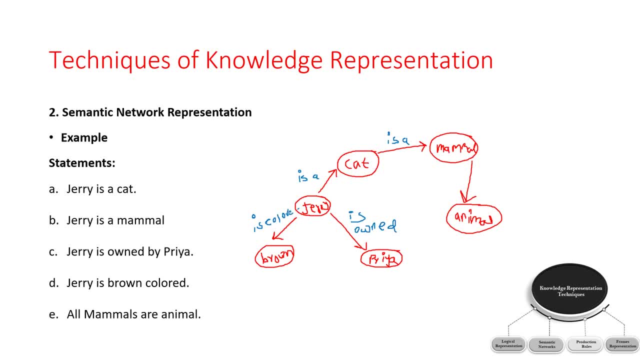 So��ar shh tihit kya ek aine ze arap peiveyde hi sapu color and all the mammals are animal. here also we can use: is a mammals is a animal. ok, this is a semantic network representation. so in this diagram we are: 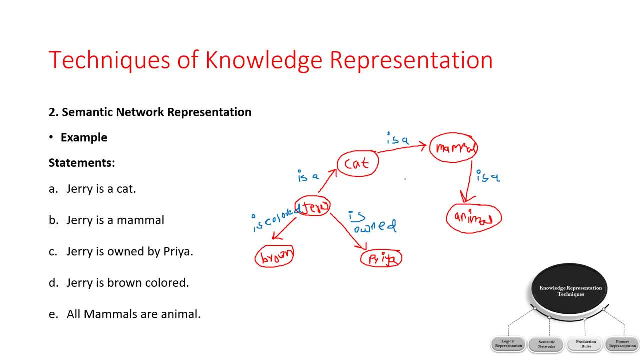 we have represented the different types of knowledge in the form of nodes and arcs, so each object is connected with another object by some relation. so drawbacks of semantic representation in the semantic network take a more computational time and a run time as we need to traverse the complete network trees. 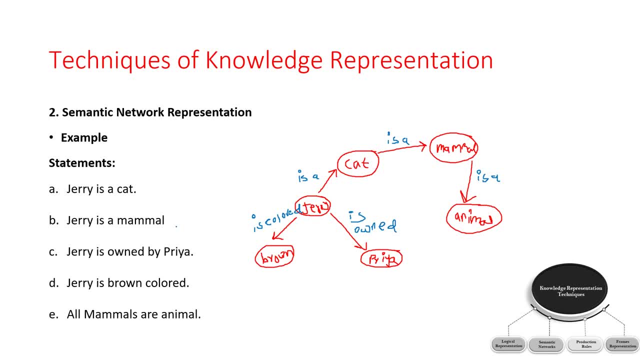 to answer some questions. so it might be possible, in the worst case scenario, that after traversing the entire tree, we find that the solution does not exist in this network. and another drawback is what this type of representations are inadequate as they don't have any equivalent quantifiers. 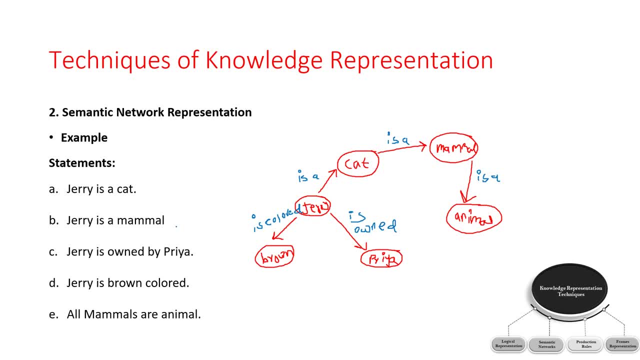 for all type, all for some and none type. so semantic network does not have any standard definition for the link, the names and this network are not intelligent and depends on the creator of the system. and what are the advantages if we use semantic network representation? so semantic networks are a natural representation of a knowledge. 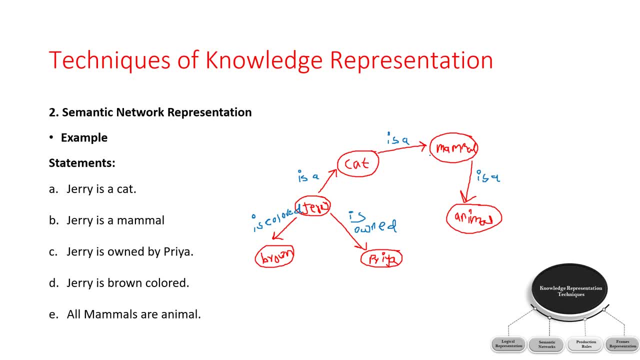 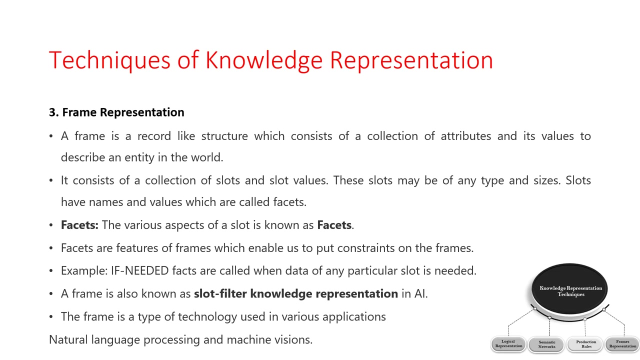 so this convey the meaning in the transparent manner and these networks are simple and easily understandable. ok, so this is a semantic network representation. so the next technique of knowledge representation is a frame representation. so frame is a record, like structure, which consist of the collection of attributes and its value to describe an entry in the world. 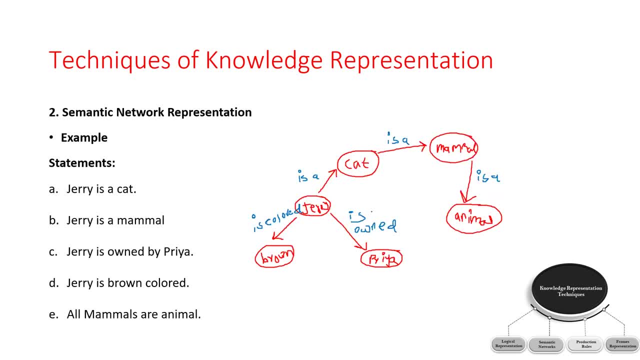 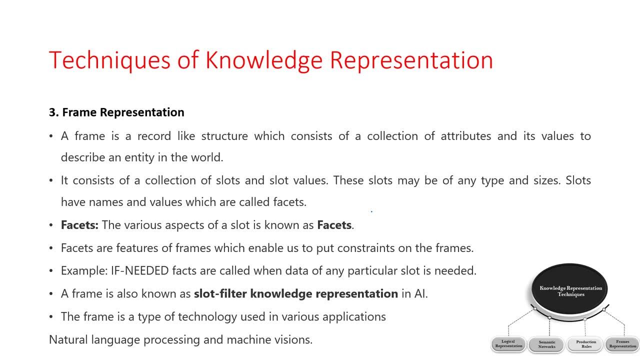 as we represent in diagrammatically or graphical form. same way, what we have to do in frame representation, we have to describe it in the form of record, like structure. ok, so frames are the AI- artificial intelligence data structure which divides the knowledge into the sub structures by representing the situations. 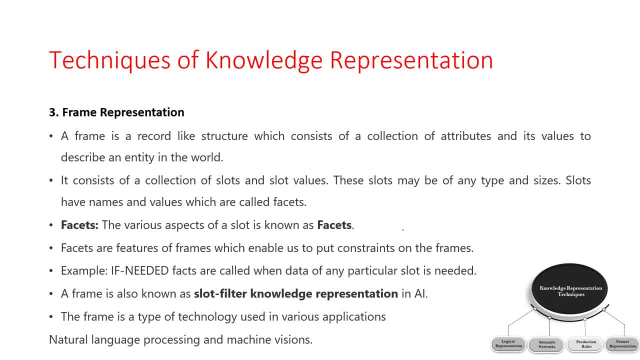 ok, so it consist of the collection of slots. the frame consist of the collection of slots and the slot values. so these slots may be of any type and size. so slots have the names and the values which are called. as a facet. whatever slots we have, it will be of any type and size. 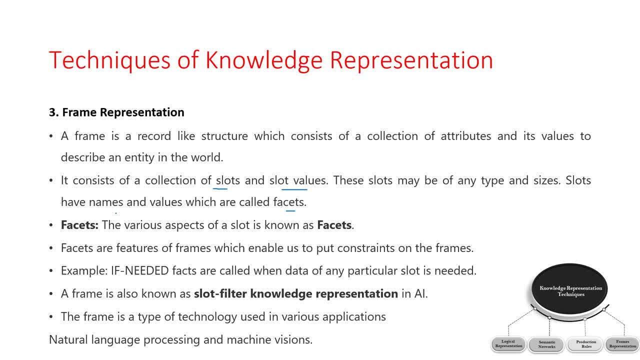 so, whatever slots we have which contain the names and values, which is called as a facet. so the facet is the various aspect of a slot, is known as a facet. so the facets are features of the frames, which enables us to put the constraints on the frame. constraint means what? 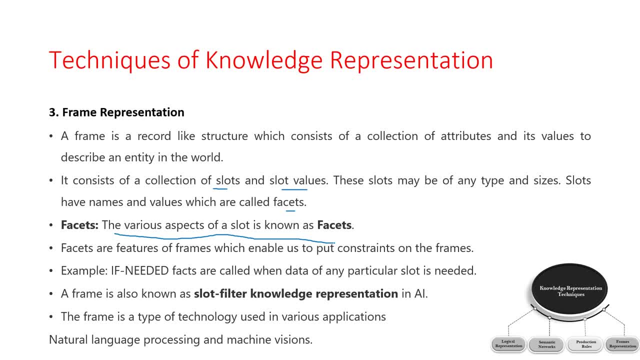 we have to providing some rules on that frame. constraint means what? providing some rules and regulations on that particular frame. so example: if needed, facts are called when the data of any particular slot is needed. ok, if needed, facts are called when data of any particular slot is a needed. 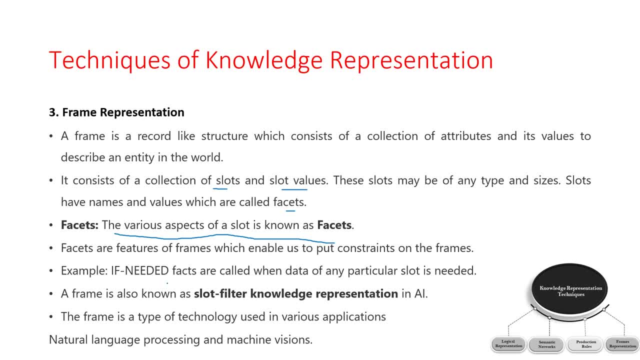 if you are having the slot is a needed. we are using the constraint here, the if needed. so so the frame may consist of any number of slots and the slot may include any number of facets and the facets may have any number of values. so the frame is also known as a slot filter. knowledge representation. 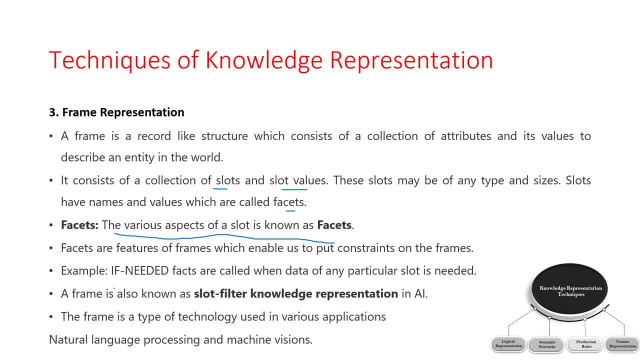 in the artificial intelligence. so these frames are derived from semantic network and later involved in our modern day classes and objects. so the single frame is not much useful. so frame system consist of a collection of frames which are connected, so in the frame the knowledge about an object or event. 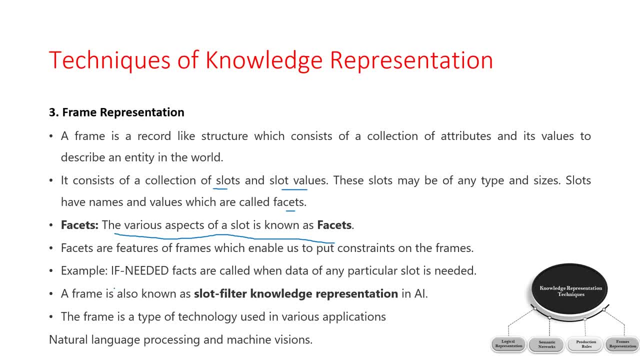 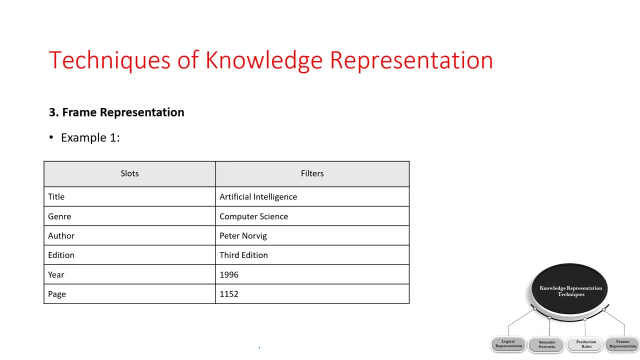 can be stored together in the knowledge base, and the frame is a type of technology which is widely used in various applications like natural language processing and the machine vision also. ok, so see, here there is one example related to the frame representation. so here let us take an example of a frame for a book. 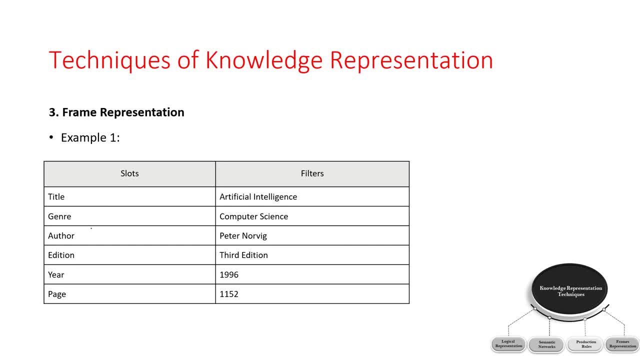 so we are having the slots like title generation, author, edition, year and pages, and the filters are artificial. intelligence is a title, generation is a computer science. author is a peter norwin. edition is a third edition, year is a 1996 and page is a 1152. 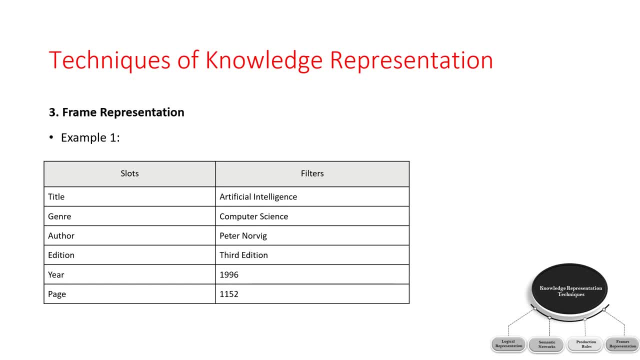 ok, so this is a frame representation. so what are the advantages of this frame representation? the frame knowledge representation makes the programming easier by grouping the related data. this frame representation is comparatively flexible and used by many applications in artificial intelligence, so it is very easy to add the slots for the new attribute and the relation. 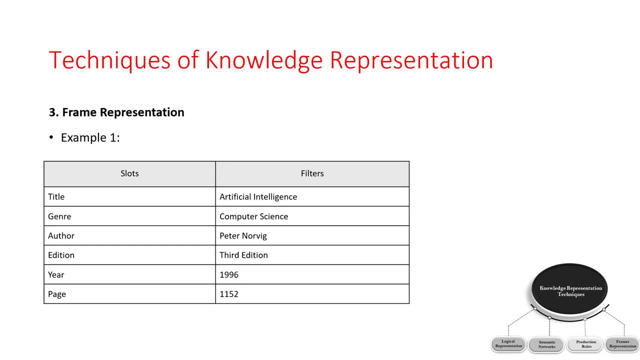 and it is easy to include the default data and to search for missing values. and the last representation is easy to understand and visualize. and what are the disadvantages of this frame representation? so in the frame system inference mechanism does not be easily proceed. inference mechanism cannot be smoothly proceeded by the frame representation. 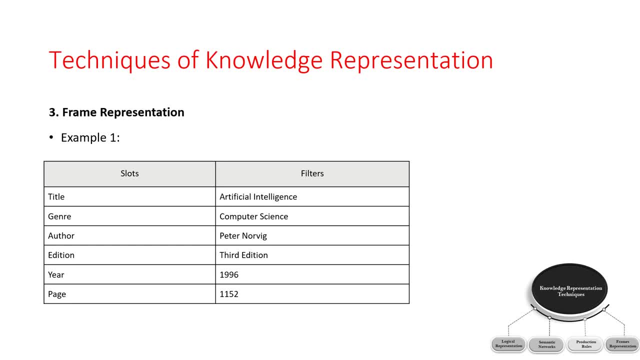 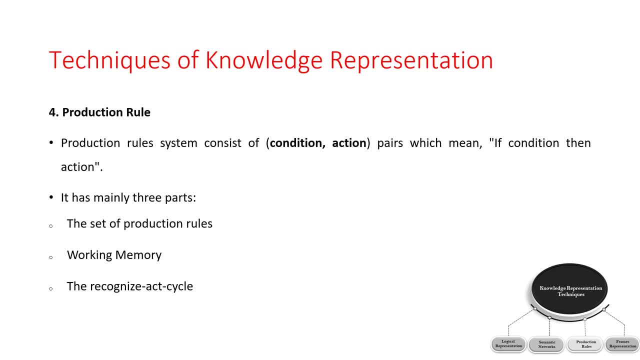 and the frame representation has a much generalized approaches. ok, so this is all about the frame representation. so the last technique of knowledge representation is the production rule. so production rules system consists of conditions and action pair, which means if condition, then action. if the particular condition is satisfied, then we will perform that action. 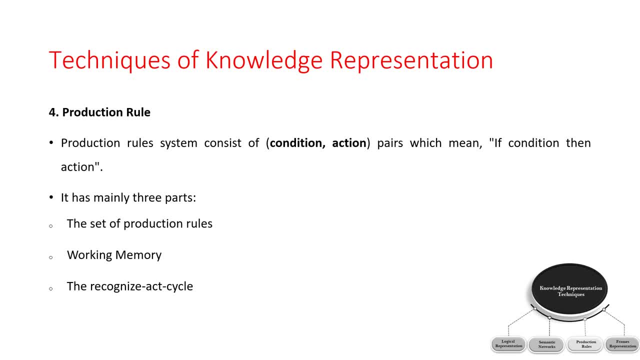 if the condition is not satisfied, then we will not perform that action. so this is a production rule. so these production rules mainly contains the three parts: first is the set of production rule, the second thing is the working memory and third thing is the recognize the act cycle. 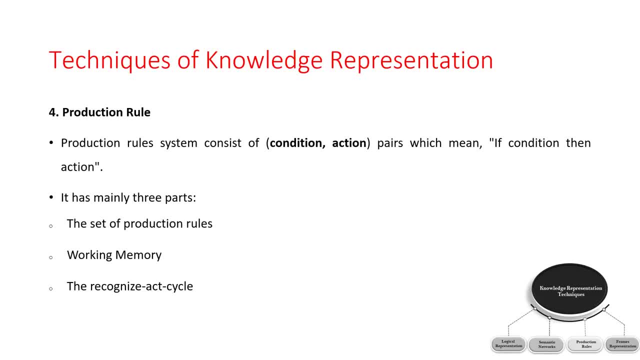 so in the production rule itself, the decision checks for the condition. if the condition exist, then production rule fires and corresponding action is carried out. so this condition part of a rule, ok, so this condition, part of the condition, part of the rule, determine which rule may be applied to a problem. 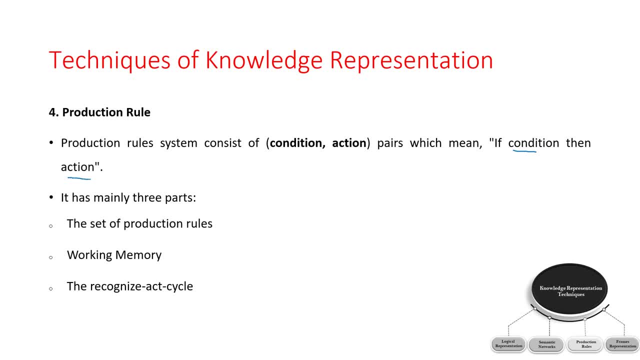 and the action part. action part carries out the associated problem solving steps. so this complete process is called as a recognize act cycle. so the working memory contain the description of the current state of the problem solving and rule can write knowledge to the working memory so this knowledge match and may fire other rules. 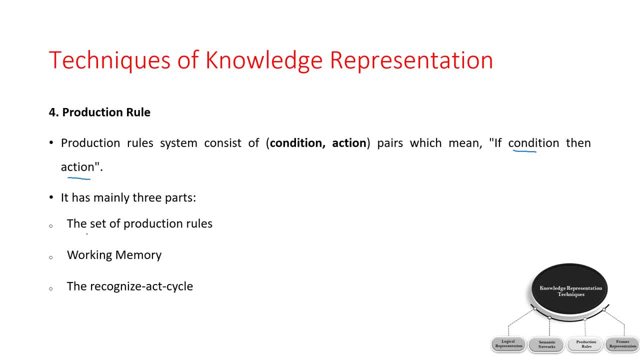 ok, and if there is a new situation which is called as a state, a situation generate- that means state generate- then the multiple production rules will be fired together. so this is called as a set of production rule. so if there is a new situation generates, then the multiple production rules will be fired together. 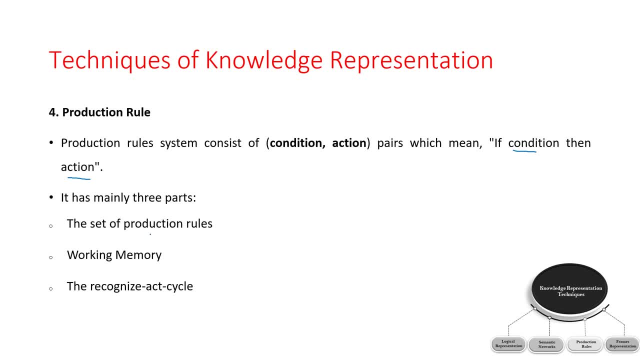 so this called the conflict set. ok, So in this situation the agent needs to select the rule from these sets and it is called as a conflict resolution. So these are the mainly three parts of the production rule. First is the set of production tool. 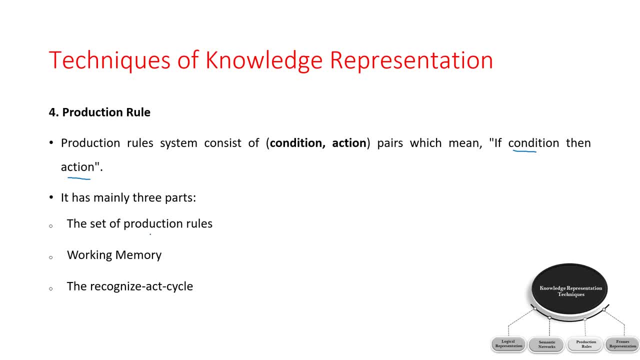 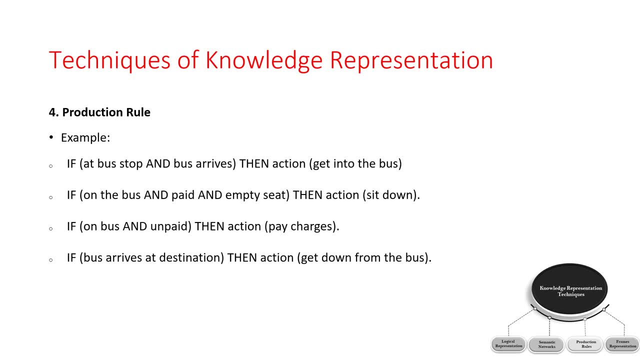 Second one is the working memory and third one is the recognize the act cycle. So see, here there is a different examples of production rule. If at bus stop and bus arrives, then action get into the bus If this condition is satisfied, as I said here, the production rule containing some conditions, 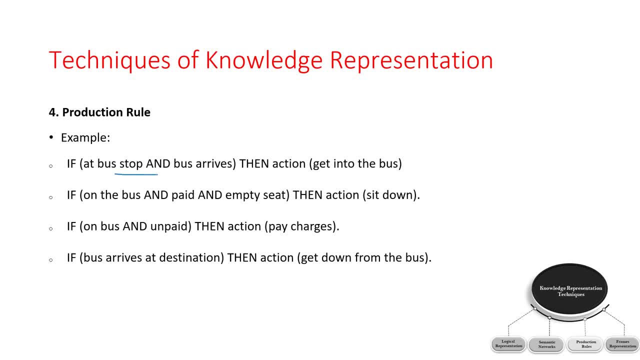 and action. So if we are having this condition, then we are performing this action. If at bus stop and bus arrives, then action: get into the bus. The second statement is: if on the bus and paid and empty seat, Then action is a sit down.